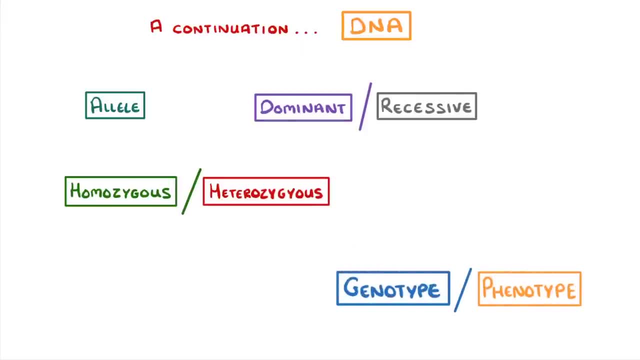 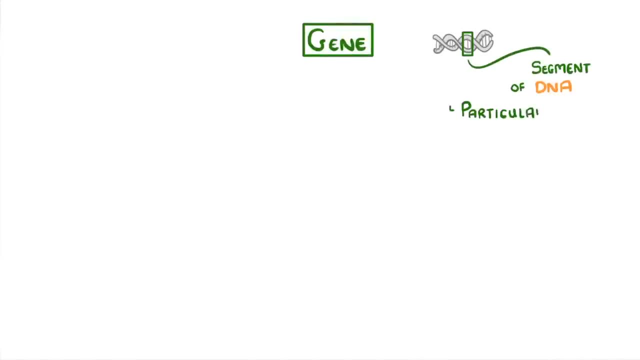 and phenotype. Now, all of these terms are related to genes and, remember, a gene is just a segment of DNA that codes for a particular type of protein. Together, these genes we inherit determine the characteristics that we go on to develop, Sometimes these traits. 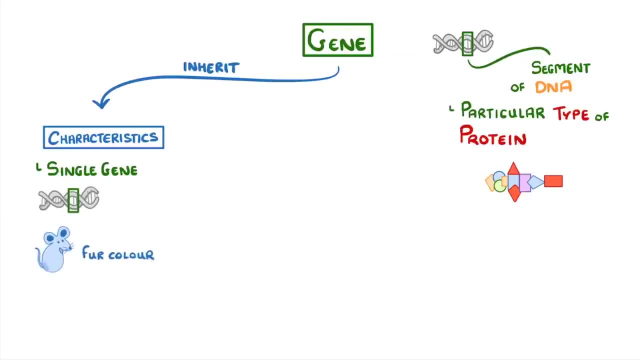 are determined by a single gene, like the ones that code for fur colour in mites and red-green colour blindness in humans. More often, though, our characteristics are determined by several different genes that interact with each other, For example, a gene that codes for a particular type of protein and a gene that codes for 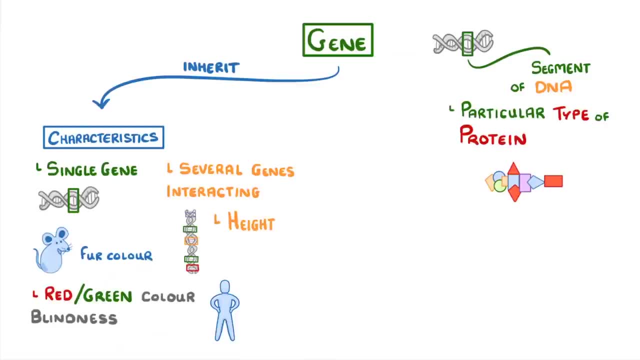 a particular type of protein, Or there are loads of genes that code for height, which is one of the reasons why we're all different sizes. If we look back at the definition of a gene, you will notice that it codes for a particular type of protein. The reason I say type of protein is that there are often multiple forms. 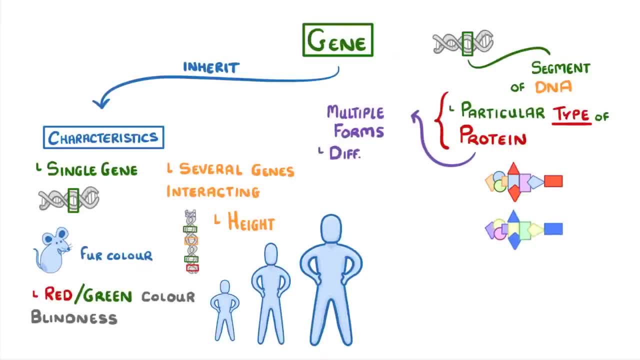 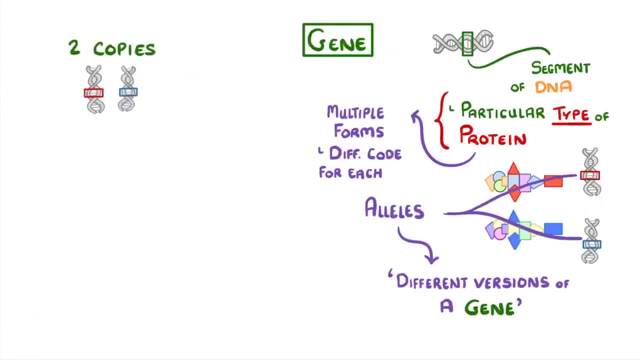 of the same protein, and so there will be a different genetic code for each of those forms, And we call these different codes alleles. So you can think of alleles as the number of different versions of the same gene, Because we have two copies of every gene, one from each of our parents. it means that 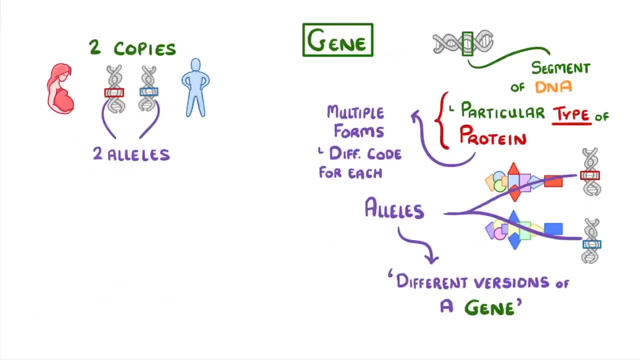 we'll have two alleles of each gene, And these could both be the same allele or they could be two different alleles. If they were the same, we'd say that we're homozygous for that allele, Whereas if they were different we would be heterozygous. 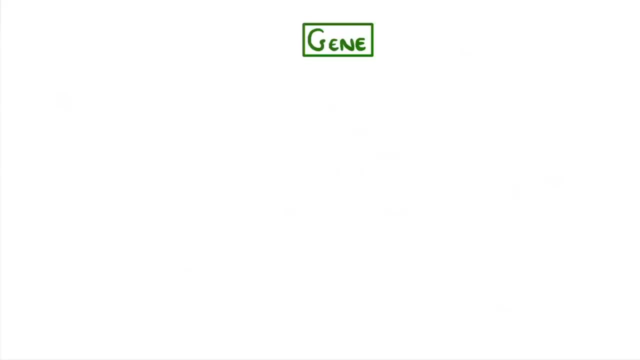 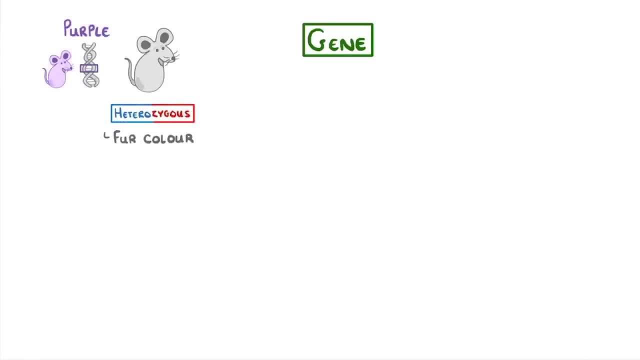 colour. with one allele coding for purple fur and the other for green fur, what colour would our mouse be? Well, it's not going to be a mix of the two. Instead, one of the alleles will be dominant and the other one will be recessive, and it's always the dominant.